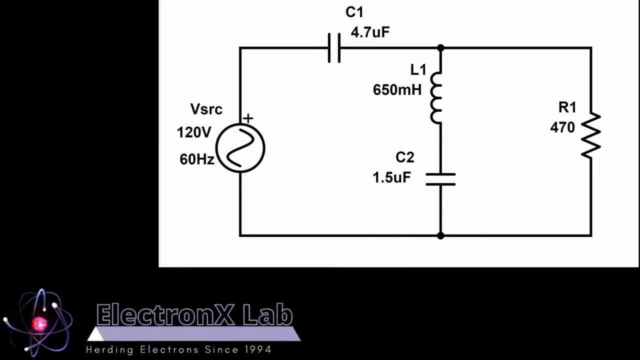 In this video I'm going to analyze this AC circuit to determine the voltage across and the current through every component. Now, this is a circuit with a combination of parallel and series components, so there will be a few more steps in this circuit analysis than there were. 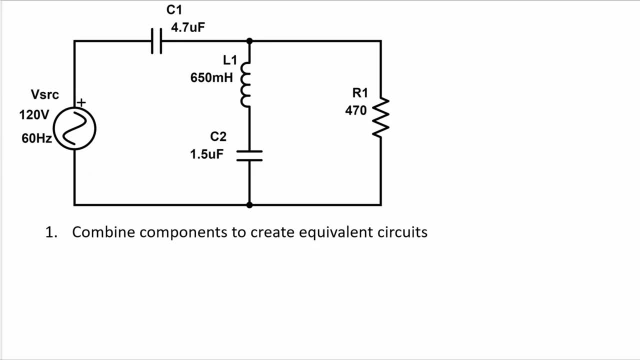 with the purely series and purely parallel circuits. The general strategy that I'm going to take is to start by combining components to create an equivalent circuit and continue combining components until circuit is one equivalent component, Then calculate voltage and current for the circuit with one equivalent component And then finally expand the circuit. 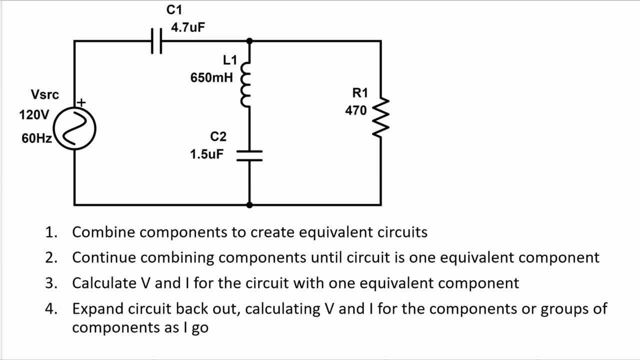 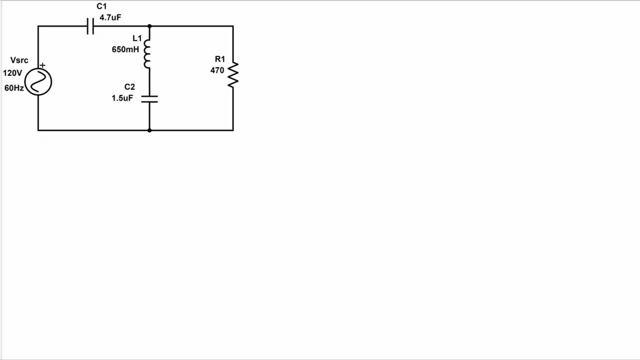 back out calculating voltage and current for the components or the groups of components as I go, until I've done this for every component in the circuit. So, more specifically to the circuit that I'm analyzing, I'm going to start by determining the impedances of each of the components here. 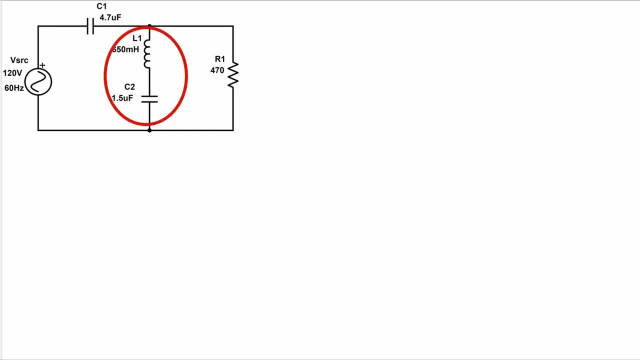 then begin combining components to create equivalent circuits. So to start, I will take this inductor and capacitor. combine them together to create this equivalent circuit. then take these two components, combine them together to create this equivalent circuit. then combine these two components together to create this. 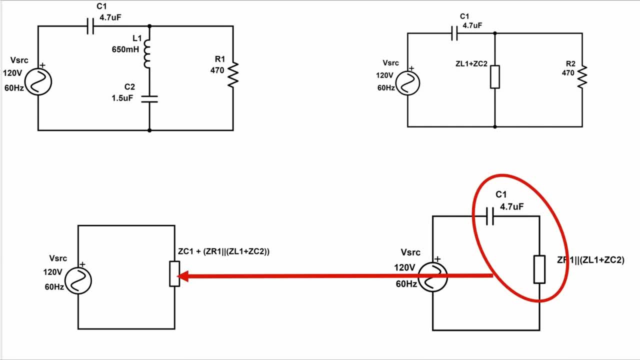 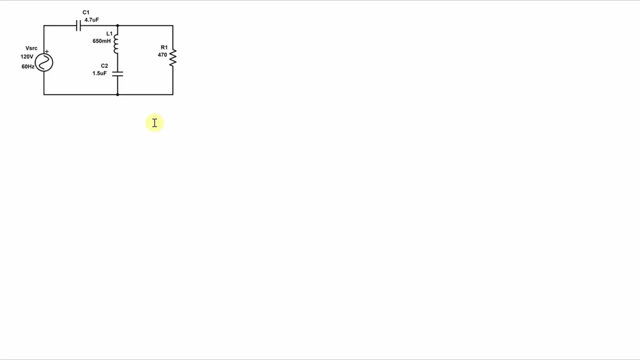 equivalent circuit with a single equivalent impedance, Then I can calculate the current in the circuit and use that information to go back to the previous equivalent circuit to calculate voltage and current and continue until I am back to the original circuit and have all the voltages and currents calculated. Now here we are with the circuit and I'll start. 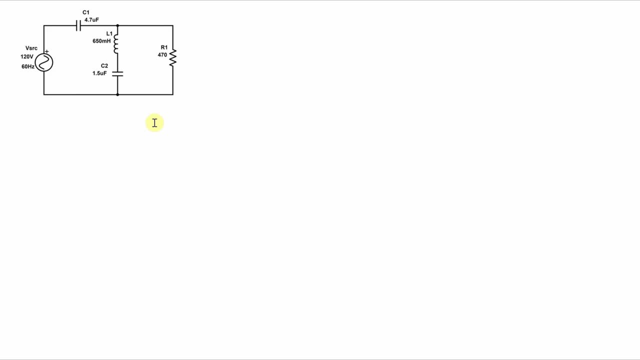 by calculating the impedances of all the components. Now, I should note that for some of the calculations, I am going to fast forward through them, So if you need to see exactly what I'm doing for each step, then you can pause the video whenever you need to. Okay, let's start with the capacitor. 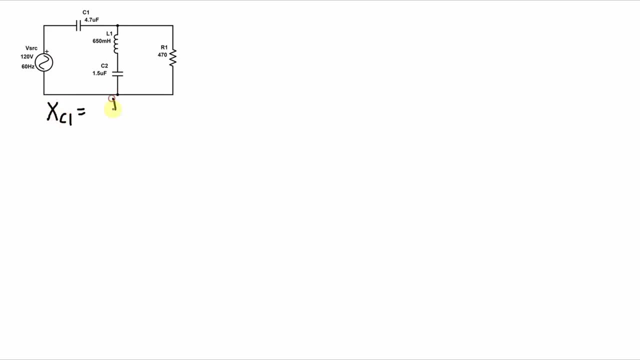 The reactance of the capacitor- capacitor 1, is 1 over 2 pi fc. The reactance of capacitor 2 has the same equation, but it is a 1.5 microfarad capacitor And the reactance of the inductor is 2 pi fL. frequency of 60 Hz. inductance of 650 millihenries. 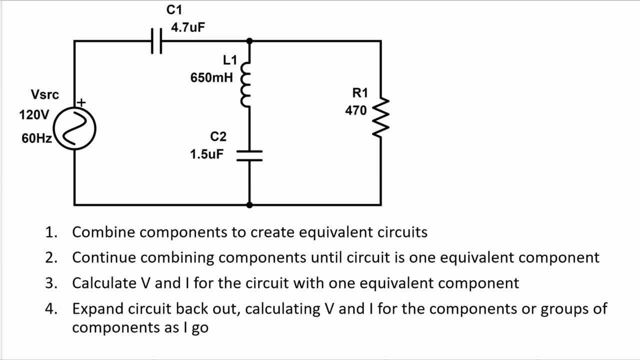 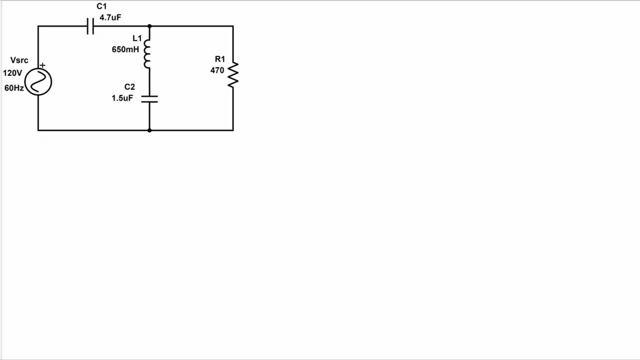 back out calculating voltage and current for the components or the groups of components as I go, until I've done this for every component in the circuit. So, more specifically to the circuit that I'm analyzing, I'm going to start by determining the impedances of each of the components here. 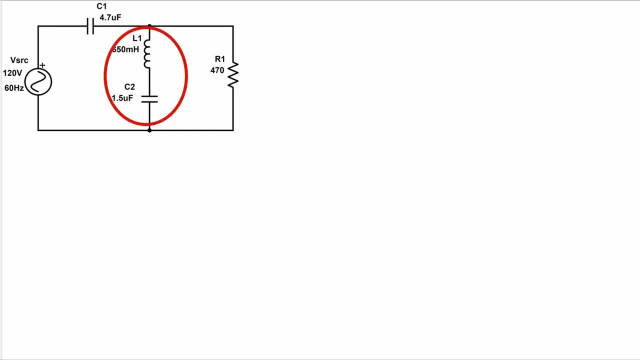 then begin combining components to create equivalent circuits. So to start, I will take this inductor and capacitor. combine them together to create this equivalent circuit. then take these two components, combine them together to create this equivalent circuit. then combine these two components together to create this. 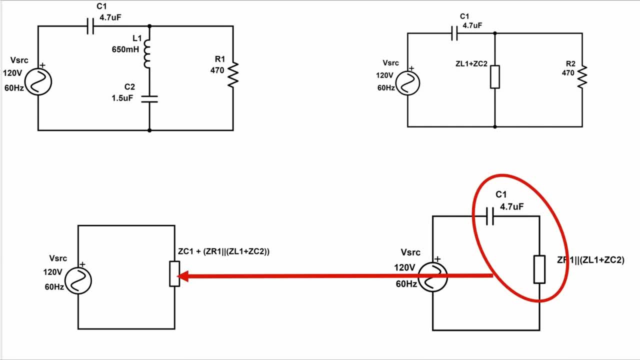 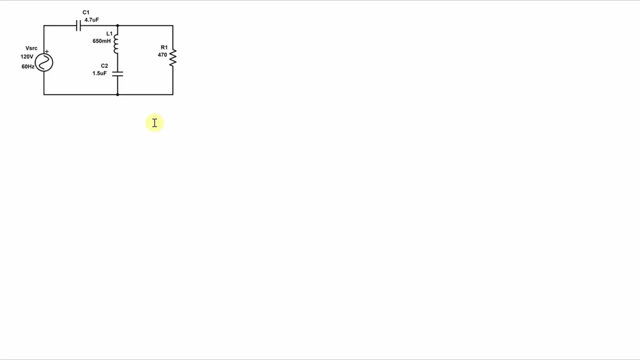 equivalent circuit with a single equivalent impedance, Then I can calculate the current in the circuit and use that information to go back to the previous equivalent circuit to calculate voltage and current and continue until I am back to the original circuit and have all the voltages and currents calculated. Now here we are with the circuit and I'll start. 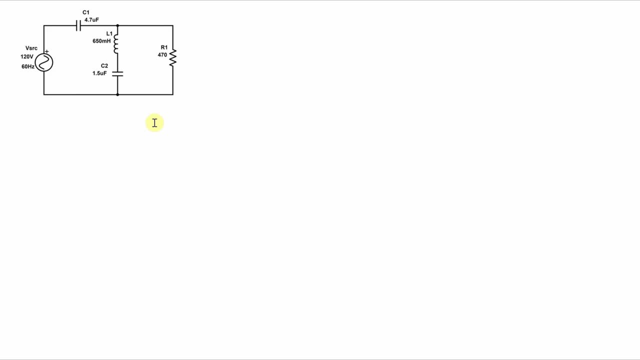 by calculating the impedances of all the components. Now, I should note that for some of the calculations, I am going to fast forward through them, So if you need to see exactly what I'm doing for each step, then you can pause the video whenever you need to. Okay, let's start with the capacitor. 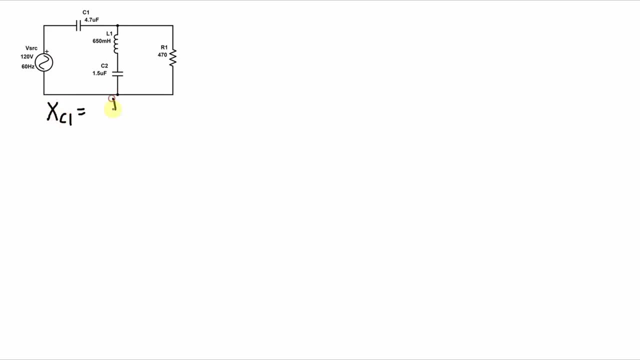 The reactance of the capacitor- capacitor 1, is 1 over 2 pi fc. The reactance of capacitor 2 has the same equation, but it is a 1.5 microfarad capacitor And the reactance of the inductor is 2 pi fL. frequency of 60 Hz. inductance of 650 millihenries. 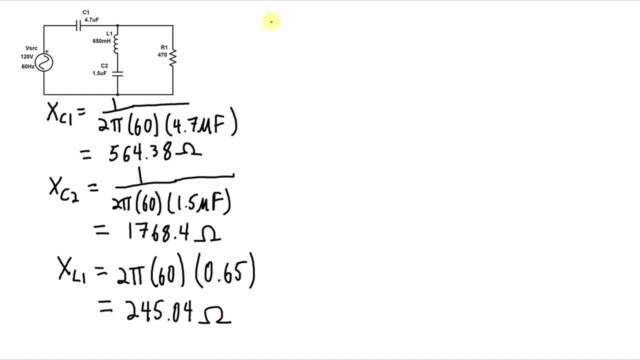 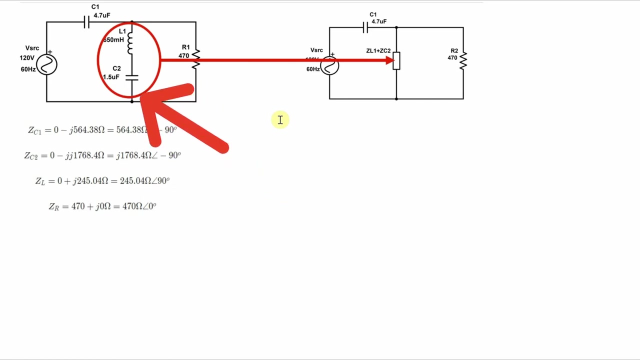 And now I can take all of these reactances and write them out as impedances. so include the phase shifts that the components will introduce. And now I'll do the calculation for the first equivalent circuit. So this is combining these two components together to give me this equivalent component. 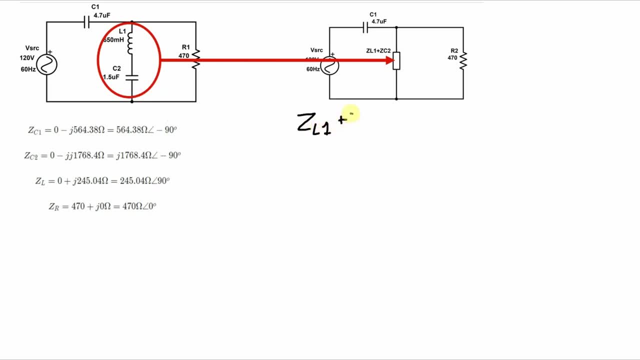 So that ZL1 or ZL1 plus ZC2, that's equal to J245.04 ohms minus J1768.4 ohms. So the effect of the reactance equation on the capacitor is going to be 1 over 2 pi fc. 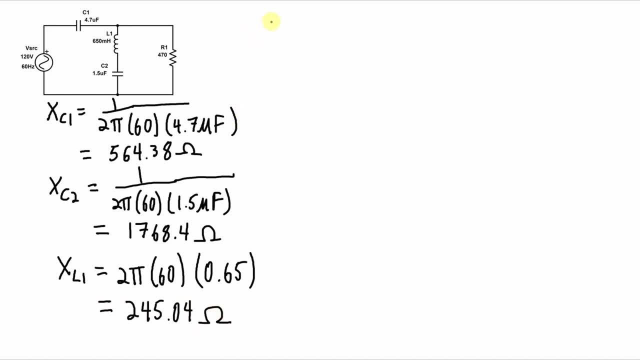 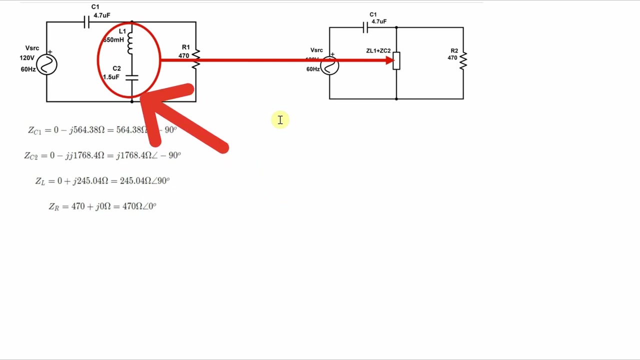 And now I can take all of these reactances and write them out as impedances. so include the phase shifts that the components will introduce. And now I'll do the calculation for the first equivalent circuit. so this is combining these 2 components together to give me this equivalent component, So that ZL1 or ZL 1 plus. 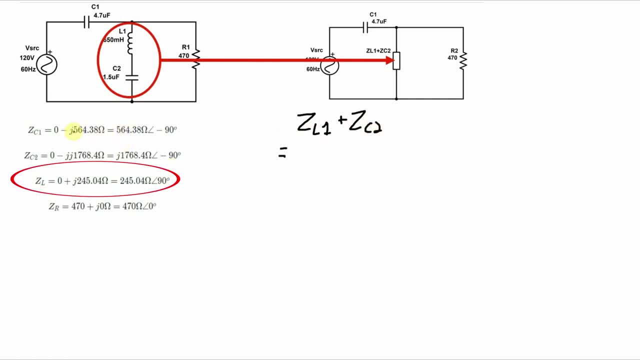 ZC 2, that's equal to J 245.04 Ohms minus J 1768.4 Ohms, Minus J 1,AMи, Minus J 2,128.ə. Minus J 428.. Minus J 1,きn. 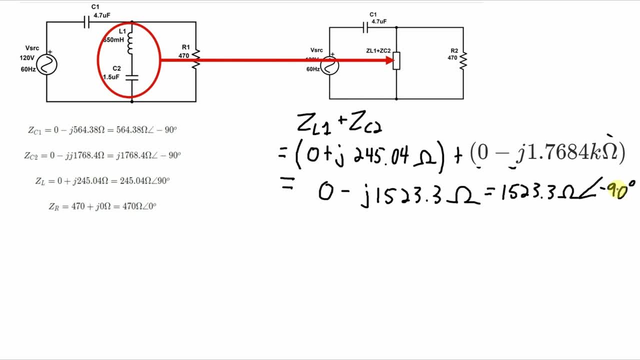 adding the impedance of the inductor plus the impedance of the capacitor gives us something that looks like a capacitor, because it's introducing this phase angle of minus 90 degrees, or it's got a negative j component. The next thing to do is combine these two components together. 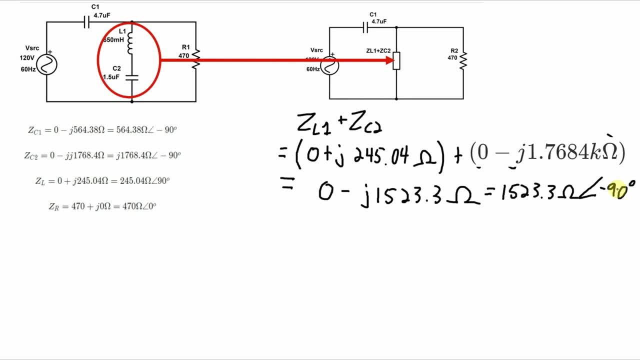 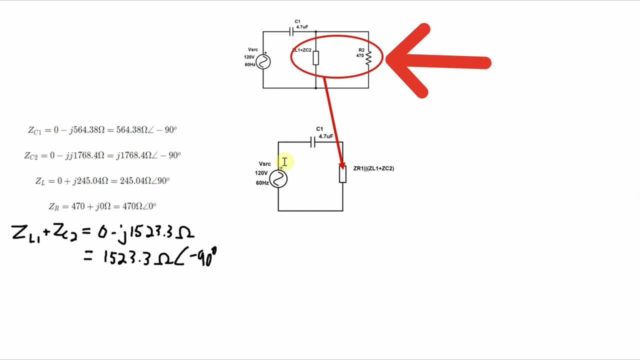 adding the impedance of the inductor plus the impedance of the capacitor gives us something that looks like a capacitor, because it's introducing this phase angle of minus 90 degrees, or it's got a negative j component. The next thing to do is combine these two components together into this one equivalent component. 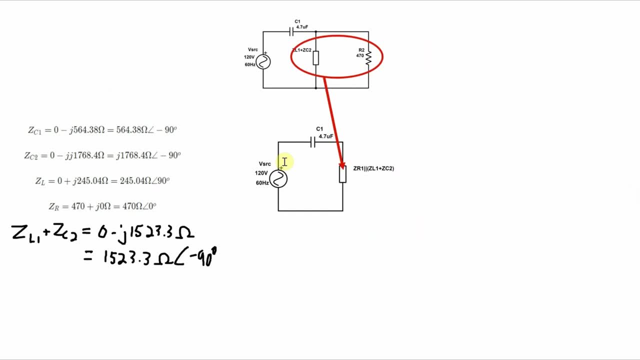 into this one equivalent component. So we've got R2 in parallel with the series combination of of inductor 1 and capacitor 2.. Now I'll convert this value, that's in rectangular coordinates, into polar coordinates. I won't go through all the steps, I'm just going to give you the value. 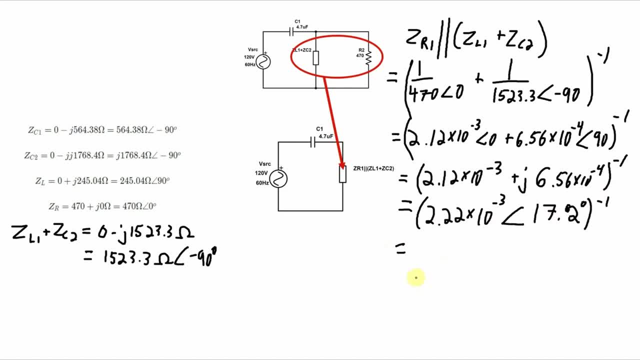 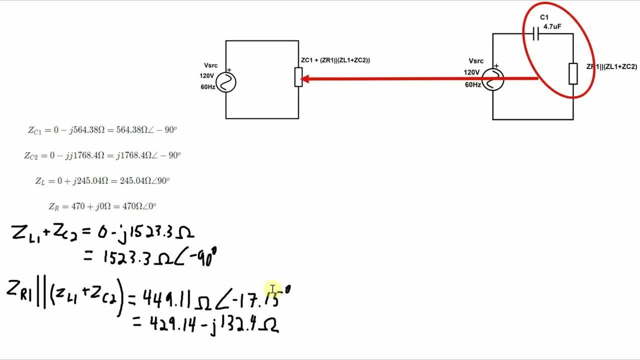 And then take the inverse of that number to give me the final impedance. Now, finally, let's make this third equivalent circuit, where we have reduced this circuit down to one equivalent impedance, by adding this capacitor 1, the impedance of capacitor 1, to this combined impedance that we've just calculated. 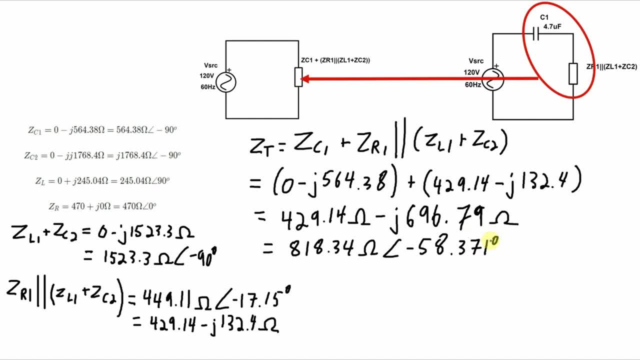 Okay, now we've got that total impedance calculated and we've got it shown here in rectangular as well as in polar. So now we've got this third equivalent circuit where we have polar coordinates, And now that we have the total impedance calculated, we can now calculate the 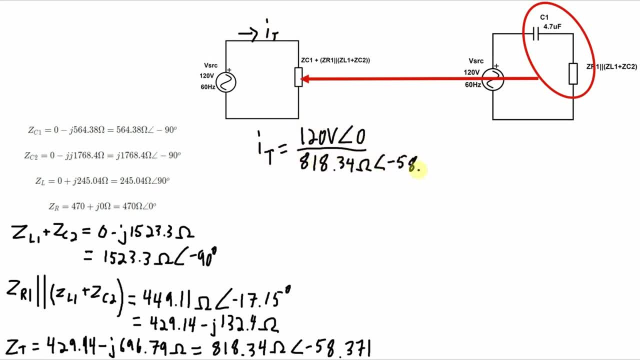 total current. Now, working backwards from this third equivalent circuit to the second equivalent circuit, IT goes through both of these components, So we can use that IT value to calculate the voltage across capacitor 1, as well as the voltage across this combination of components here. 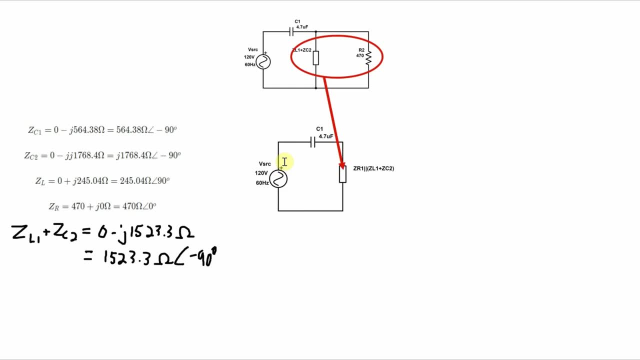 So we've got R2 in parallel with the series combination of of inductor 1 and capacitor 2.. Now I'll convert this value, that's in rectangular coordinates, into polar coordinates. I won't go through all the steps, I'm just going to give you the value. 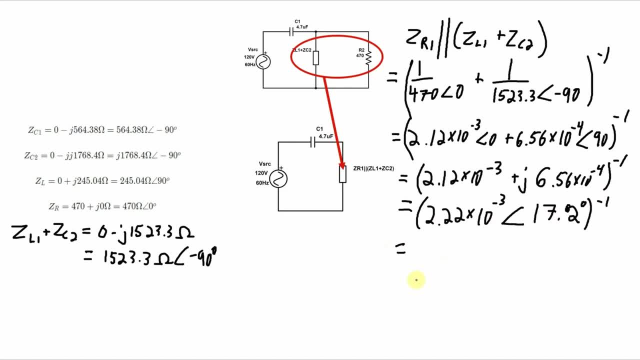 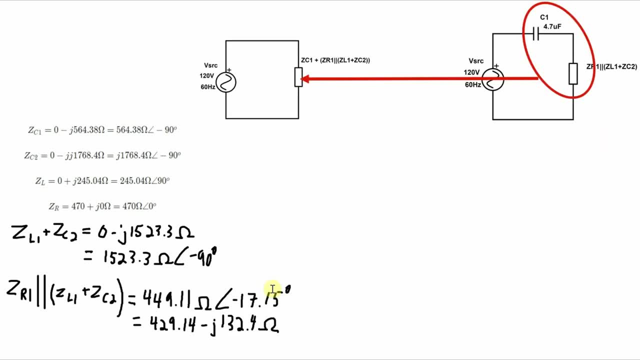 And then take the inverse of that number to give me the final impedance. Now, finally, let's make this third equivalent circuit, where we have reduced this circuit down to one equivalent Impedance, by adding this capacitor 1, the impedance of capacitor 1, to this combined impedance that we've just calculated. 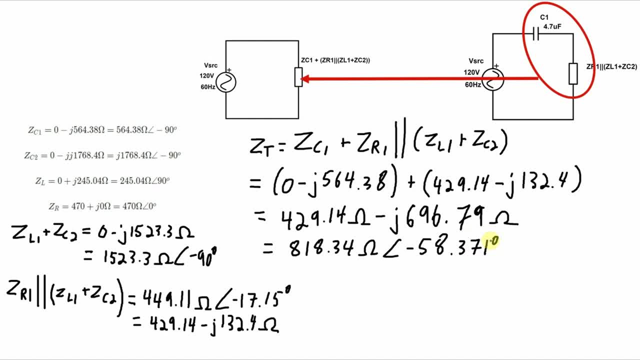 Okay, now we've got that total impedance calculated and we've got it shown here in rectangular as well as polar coordinates. And now that we have the total impedance calculated, we can now calculate the total current. So we've got R2 in parallel with the series combination of minus 90 degrees or. 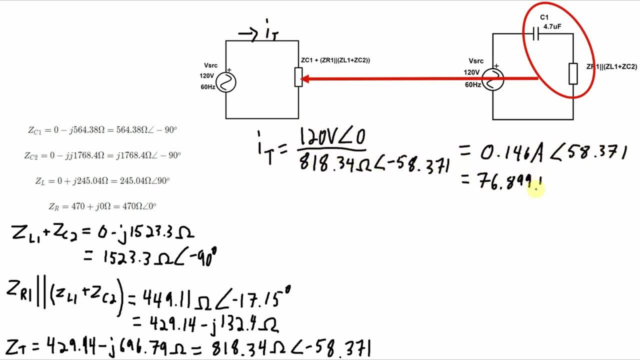 minus 90 degrees or polar coordinates, And then take the inverse of that number to give me the final impedance. And then take the inverse of that number to give me the final impedance, Now working backwards from this third equivalent circuit to the second equivalent circuit. 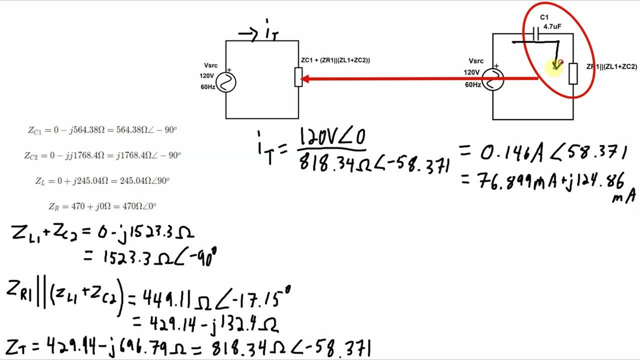 I? t goes through both of these components. So we can use that I t value to calculate the voltage across capacitor 1 as well as the voltage across this combination of components here. So that calculation is the current through capacitor 1.. So that calculation is the current through capacitor 1. 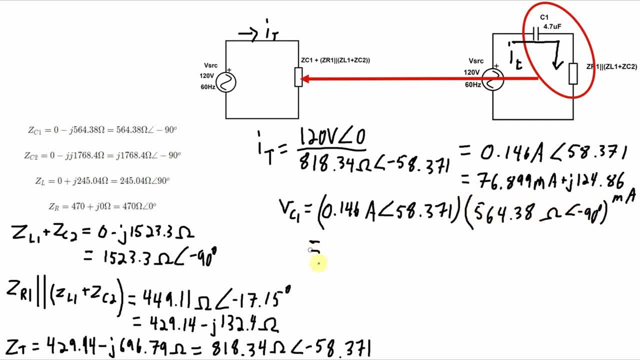 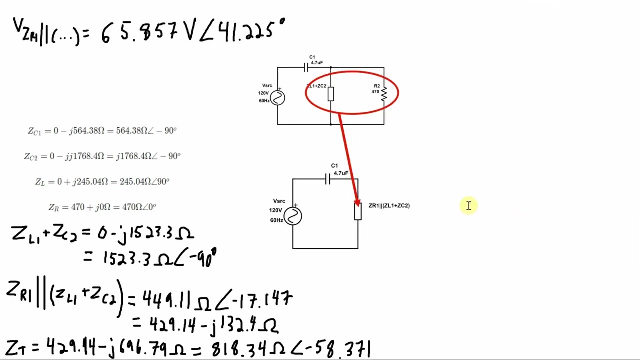 times the impedance of capacitor 1.. And in rectangular coordinates, that is- And we can do the same- basic calculation for the voltage across this combination of components. The value that I need now, going back a step from the second equivalent circuit to the first equivalent circuit, is the voltage across this combination of components. 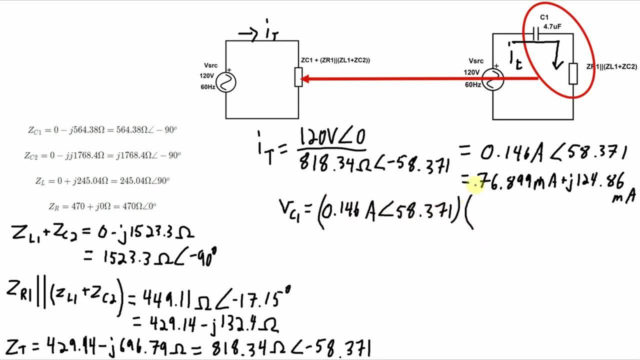 So that calculation is the current, through capacitor 1 times the impedance of capacitor 1. And in rectangular coordinates, that is, And we can do the same basic calculation for the voltage across this combination of components, The value that I need. now, going back a step from this second equivalent circuit to this first, 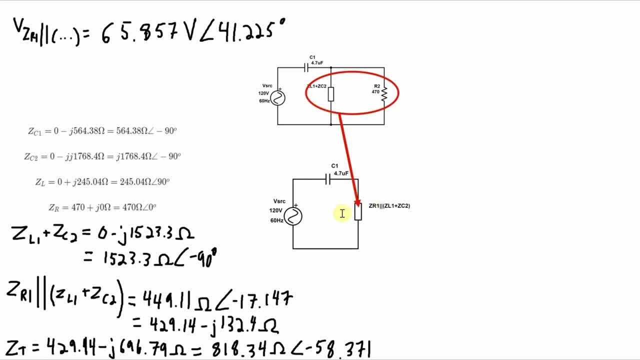 equivalent circuit is the voltage across this combination of components, the combination of R1 in parallel with L1 plus C2. And since those components are in parallel, the voltage that I've just calculated here is the same voltage across this combination of components. So that's the 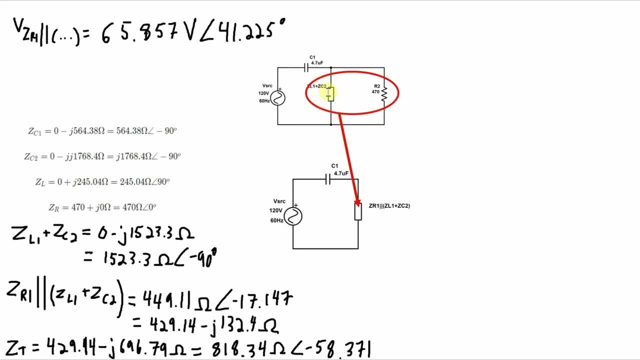 same as the voltage across L1 plus C2, as well as the voltage across resistor 2.. Although I just noticed now that that should be resistor 1, shouldn't it? So I can use that voltage to calculate the current through each one of these two components. 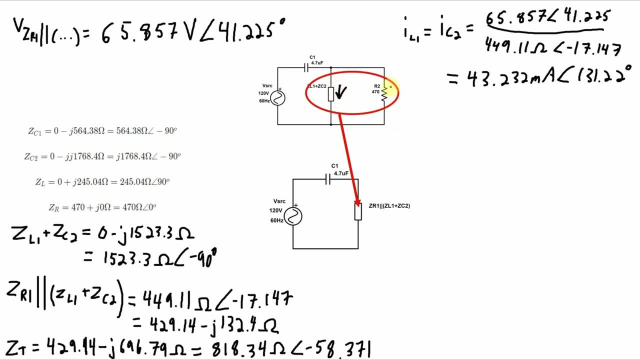 So that is that current there. Next, I can calculate this current here So that, like I said, that should be R1.. So it's the same voltage Divided by the impedance of the resistor. Now the last two values that I need are the voltage across inductor 1 and the voltage across 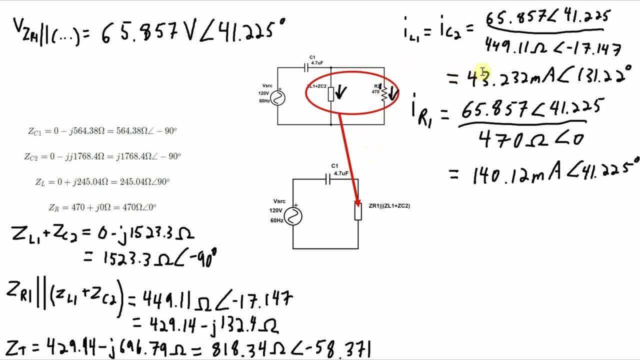 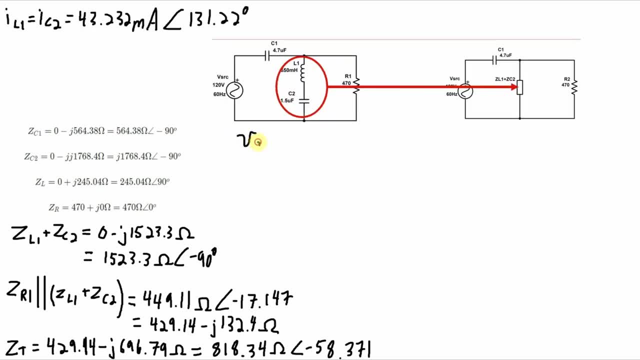 capacitor 2.. And I can use this current that I've just calculated, along with the impedance of capacitor 2 and inductor 1, to calculate those voltages. And then I'm done, And the voltage across the capacitor, Same calculation, Current times, the impedance of the capacitor. 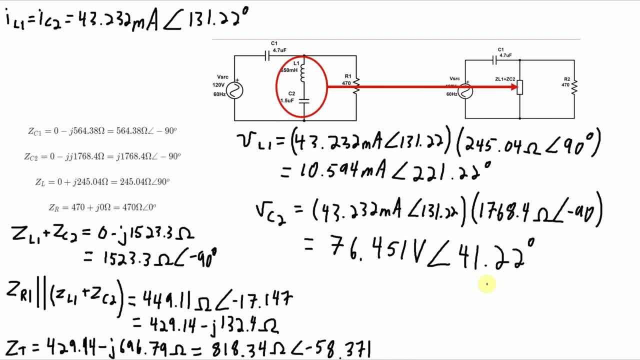 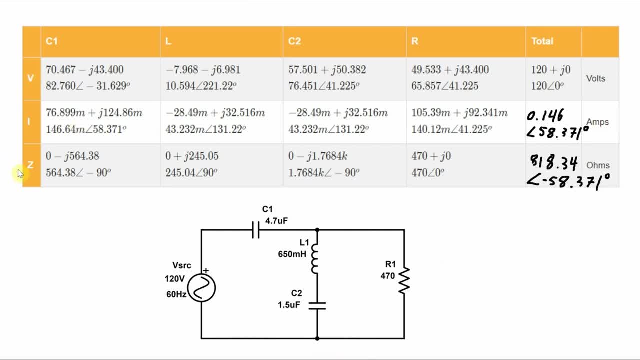 And that's it. That was the last calculation. Now here's the table with all the values. So in the table we have the voltages, the currents and the impedances for all of the components C1, the inductor, C2, the resistor, as well as the totals. Now this table and example: 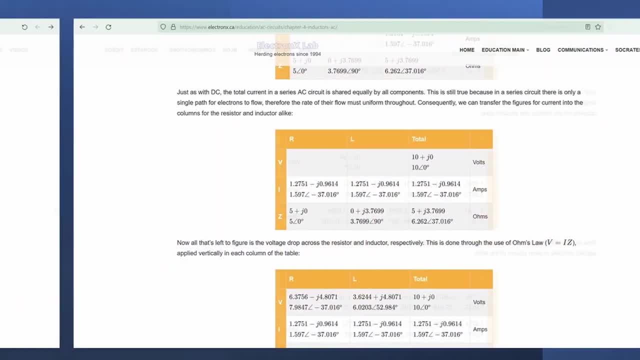 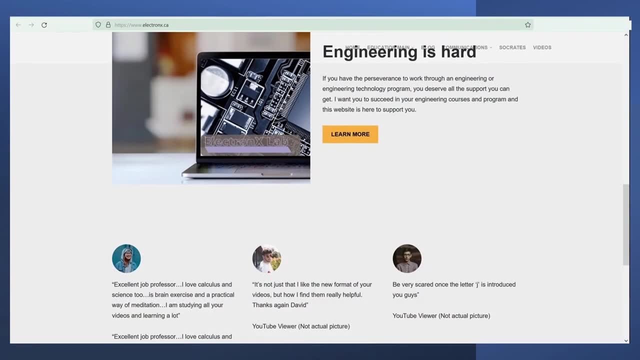 problem came up, So I'm going to use the current times- the impedance of the capacitor- And I'm going to talk a little bit about the current times. And Ogsdorff actually provider a free, open source textbook and you can find the link to the problem in the description. That website covers AC circuits DC. Ogsdorff provider a free, open source textbook and you can find the link to the problem in the description. That website covers AC circuits DC. 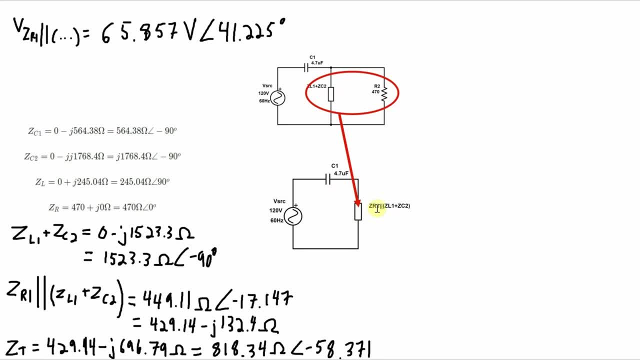 The combination of R1 in parallel with L1 plus C2.. And since those components are in parallel, the voltage that I've just calculated here is the same as the voltage across L1 plus C2, as well as the voltage across resistor 2.. 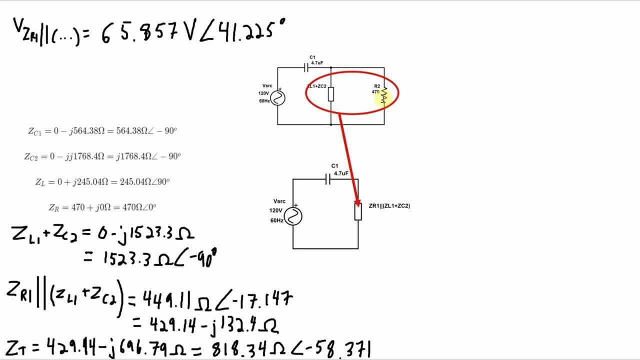 I just noticed now that that should be resistor 1.. Shouldn't it, Wouldn't it, Wouldn't it? So use that voltage to calculate the current through each one of these two components. So that is that current there. Next, I can calculate this current here, So that: 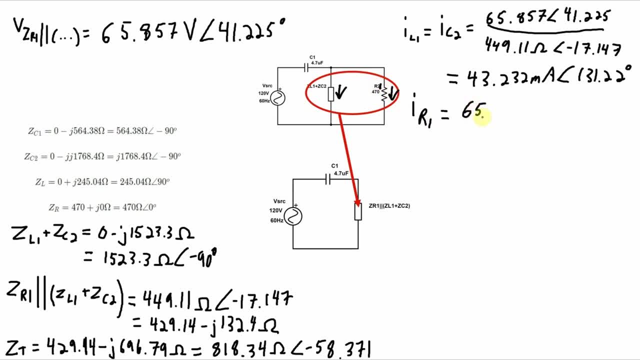 like I said, that should be R1.. So it's the same voltage divided by the impedance of the resistor. Now the last two values that I need are the voltage across inductor 1 and the voltage across capacitor 2.. And I can use this current that I've just calculated, along with: 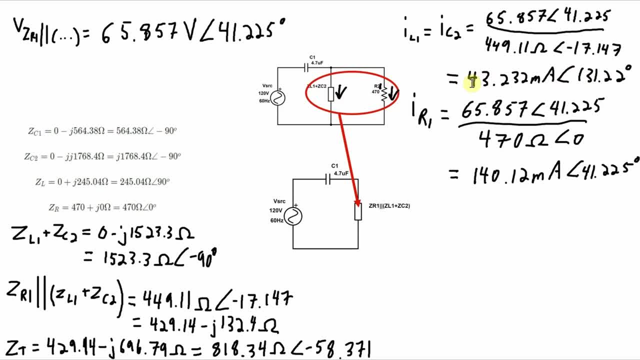 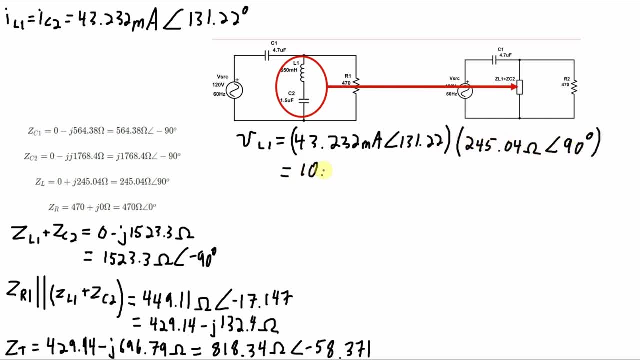 the impedance of capacitor 2 and inductor 1 to calculate those voltages. And then I'm done. And the voltage across the capacitor, Same calculation, Current times, the impedance of the capacitor. And that's it. That was the last calculation. Now here's the table with all the values. 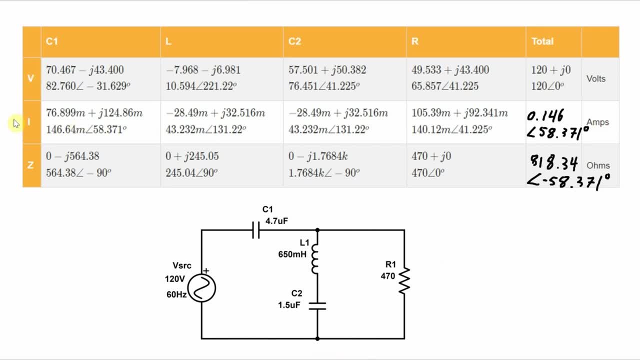 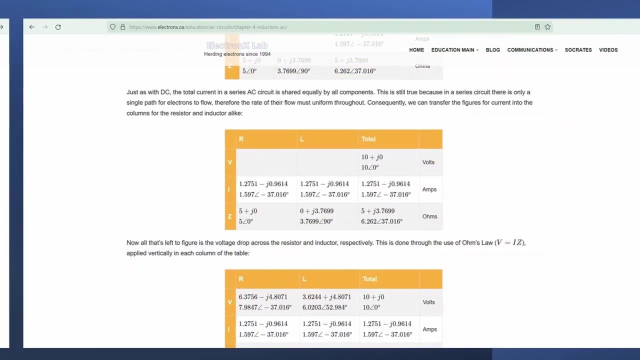 So in the table we have the voltages, the currents and the impedances for all of the components C1, the inductor, C2, the resistor, as well as the totals. Now this table and example problem came from a free, Open Source textbook and you can find the link to the problem in the description. That website covers AC circuits, DC circuits and communication systems, And if you're lucky enough to be watching this by this occasion, please say hello in the chat for that video. So I've included the link in the description of this video to the metadata. if you want to know what these components totally do, please check it out there. 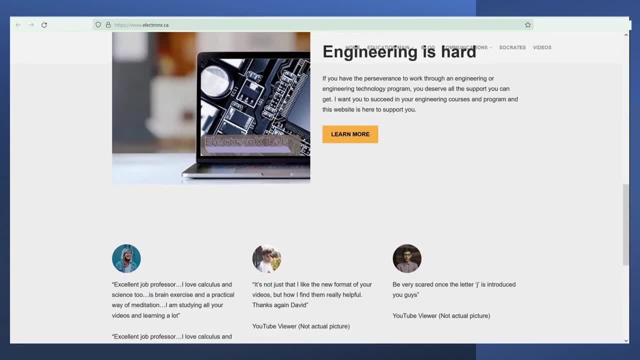 And if you're lucky enough to be a member of Channel One, buy from Secure Bears and earn money for Liang facility. Also, you can use the money we've taken from from our awesome Iranian content toUM enough to be viewing this video far enough into the future from when i created it. it will also 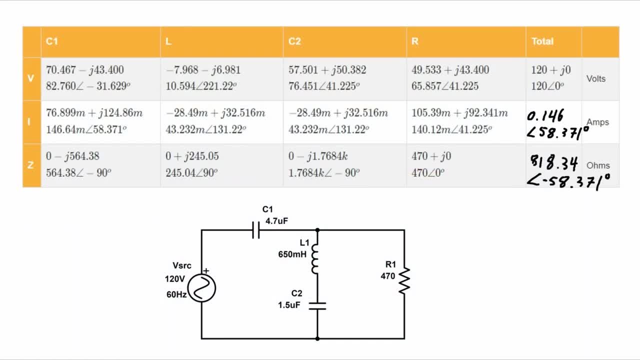 cover electronic circuits and digital electronics too. as always, thank you so much for watching. i'll see you in the next video.